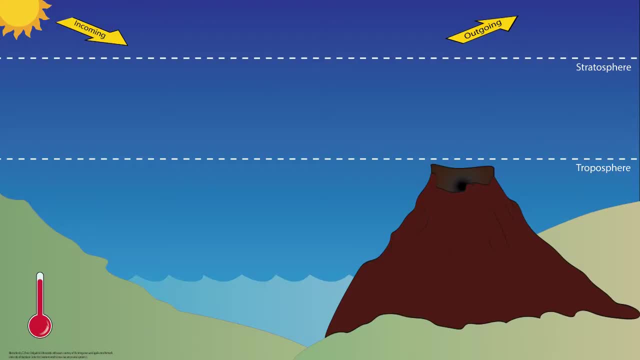 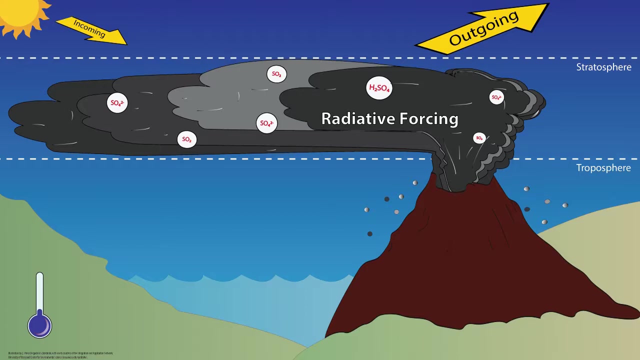 We're using volcanic eruptions because they represent rapid radiative forcing. So when an eruption occurs, aerosol, dust and different particles are injected into the atmosphere. If the eruption is really really strong, it will go into the stratosphere and once in the stratosphere it will undergo certain chemical changes and it will make an aerosol cloud. 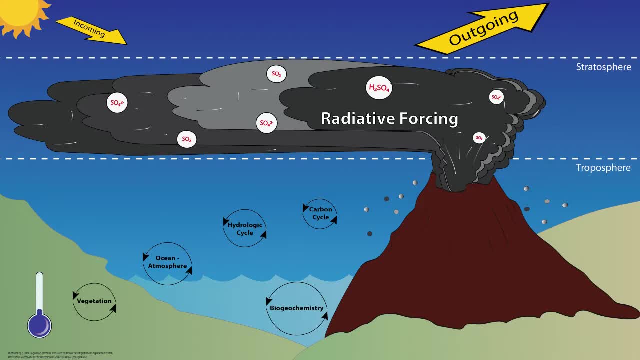 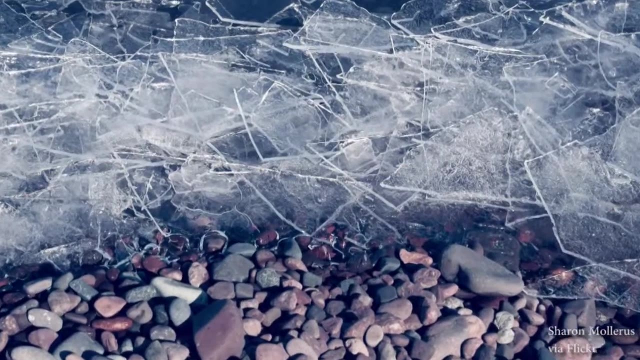 That cloud will start moving forward and it will lead to changes in temperature and vegetation and precipitation, not only in the atmosphere but also in the atmosphere. So we're looking at not only where the eruption occurred but globally as well. So after the eruption occurs we have these cooling periods, so the temperature drops and some studies have said that after the eruption occurs we can see changes in precipitation patterns. 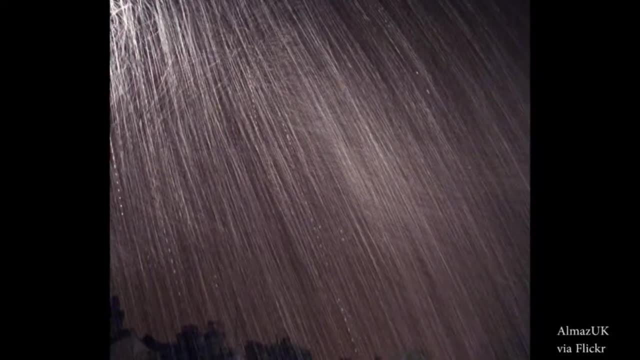 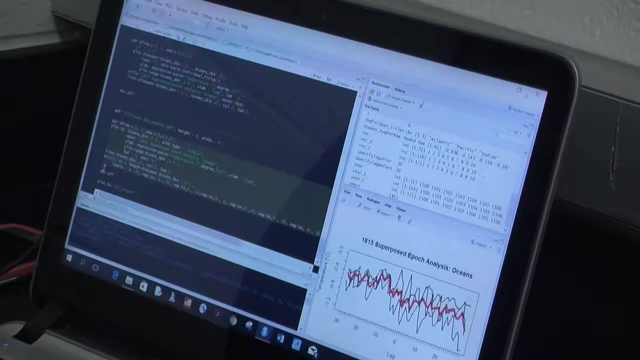 So that's one of the areas that I'm interested in is looking at how rainfall and temperature change after a really strong eruption occurs and then doing the comparison with model output. Imagine corals being like the trees. So corals are like the trees of the ocean. 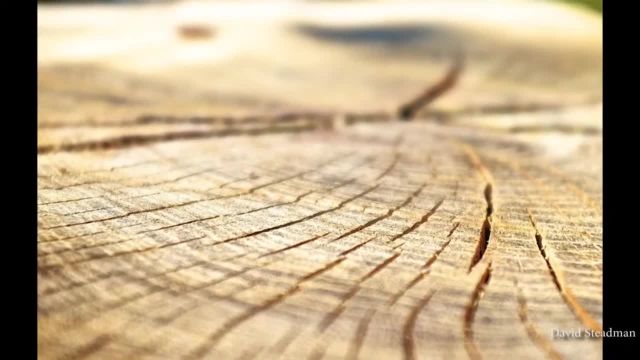 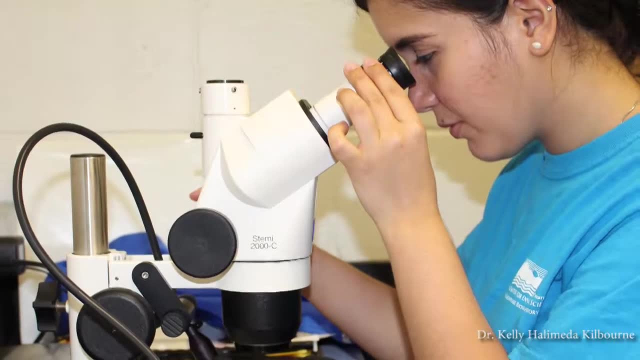 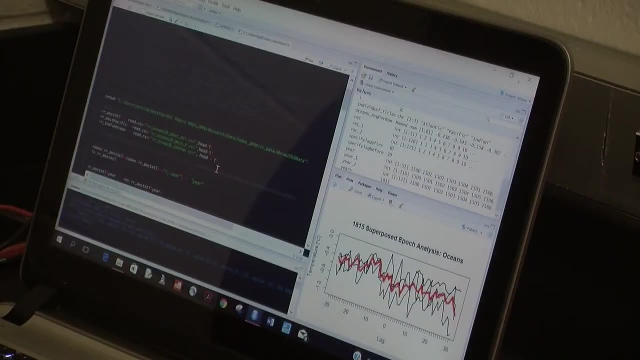 So, similar to how trees have tree rings for every year of growth, the corals pretty much do the same thing, And that way we can actually go back, study them and make reconstructions about the past and past temperatures. We use state-of-the-art Earth System models to understand the past, present and future climate. 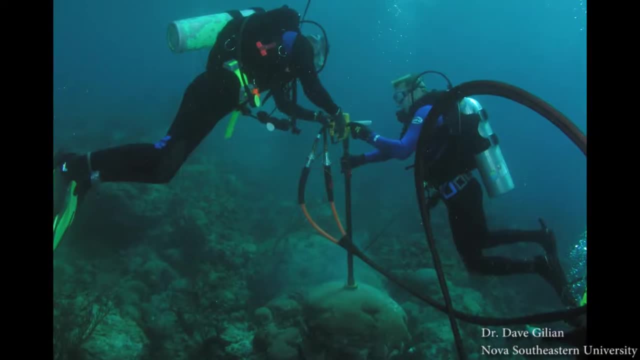 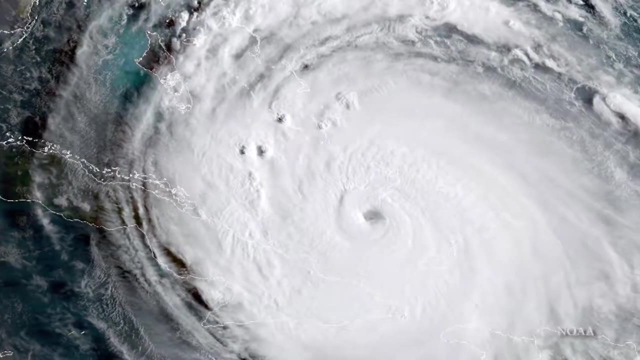 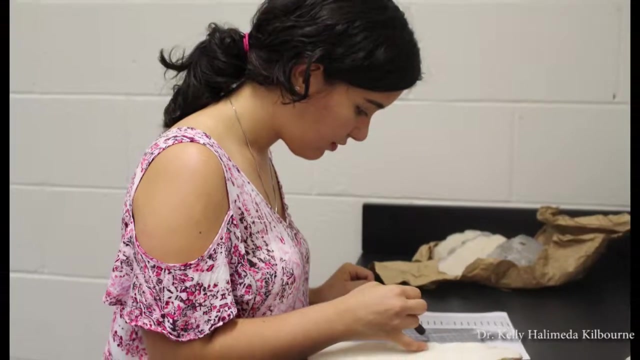 Climate models help us understand changes in sea level rise or temperature changes in different regions or globally, or globally Things such as hurricanes. where are they going? All these things are related to models. The goal of my research, basically, is just to be more confident in model predictions. 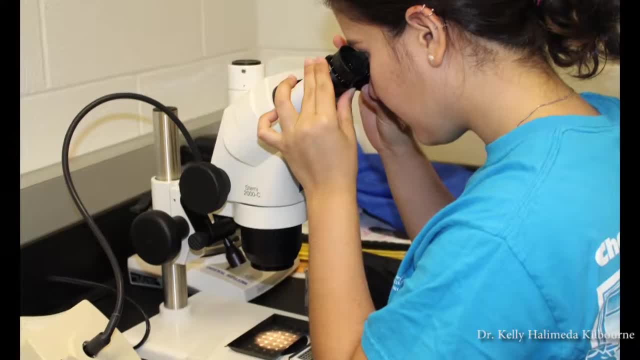 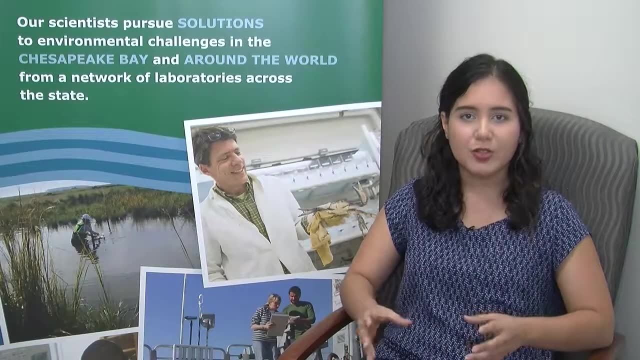 So that's why we're making these comparisons with reconstructions of past data from corals and tree rings and cave deposits, to just have a better understanding that the models are actually doing it right and that we can be more confident in what the predictions of the models are going to tell us. Subtitles by the Amaraorg community.